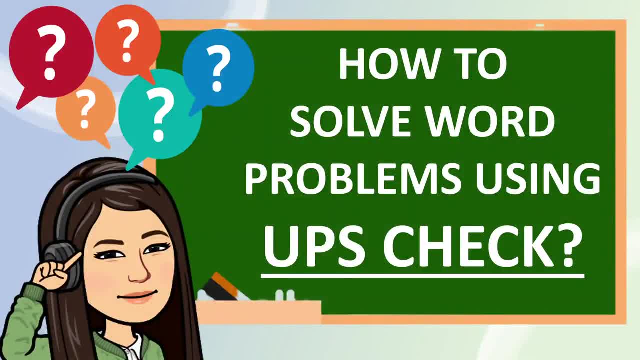 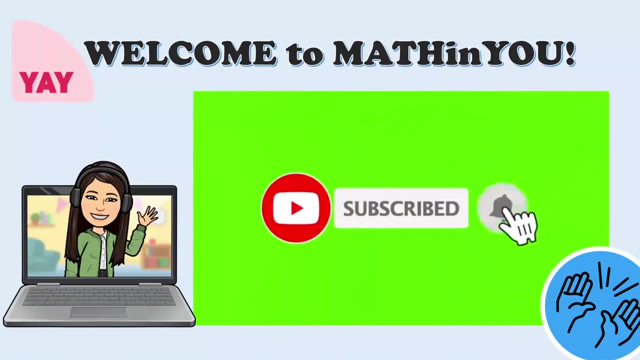 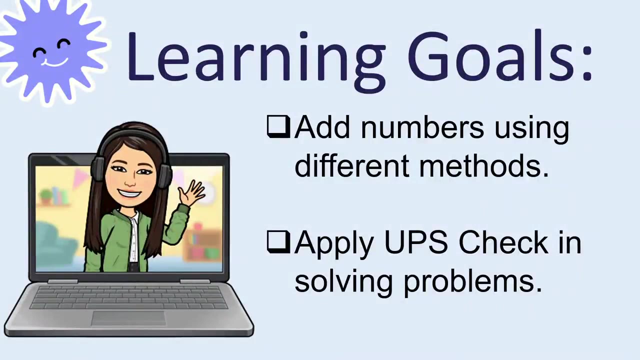 Hi everyone. Today's session is about how to solve word problems using UPS check. This is Teacher Angel, and welcome to Math in You. The learning goals of today's topic is to add numbers using different methods and to apply UPS check in solving problems. 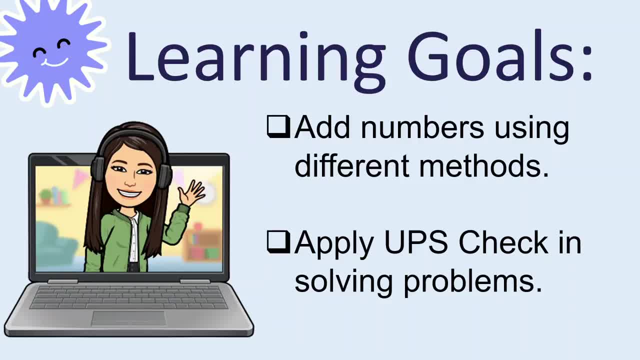 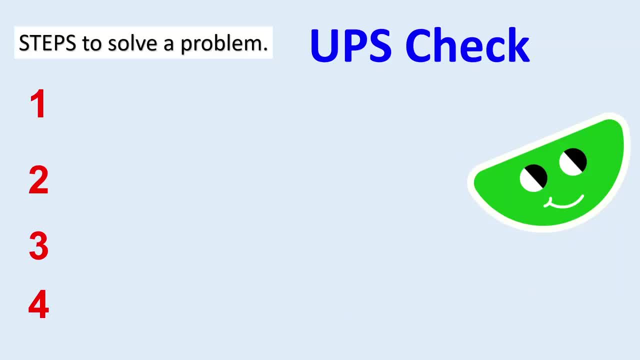 What does UPS check mean? So we can use this to solve problems. We can use this as our steps or guides in solving problems. First step, U? U means understand. You read the problem with understanding. What am I looking for? What do I know? 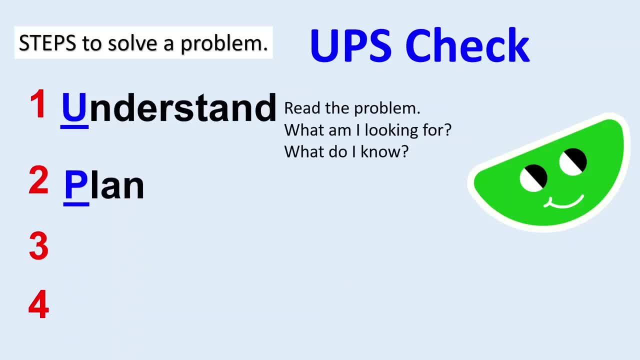 Second step is letter P plan. You choose a strategy or a method to use to solve the problem. Alright, you can draw a model. Third step is to solve. Carry out the plan In here. you will show all your words and label your answers. 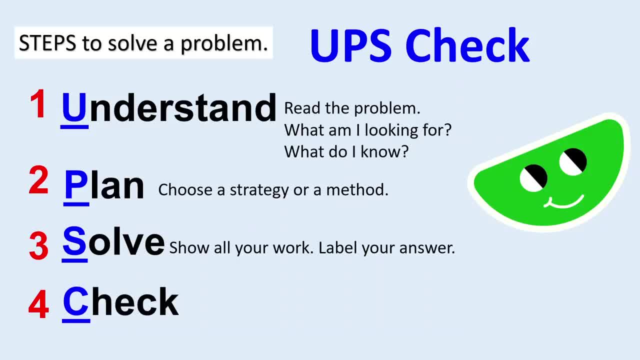 And the last step is to check, Check, Look back, Explain and justify, Identify your work and ask yourself: is your answer or is my answer reasonable? Is my answer correct? Alright, so let's apply these steps, this UPS check in solving problems. 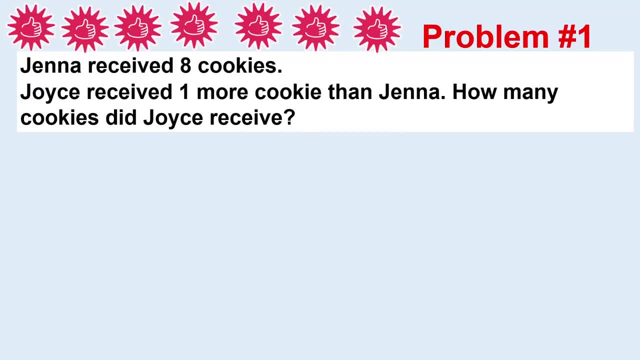 Problem number one: Jenna received eight cookies. Joyce received one more cookie than Jenna. How many cookies did Joyce receive? So the first step is to understand The problem. read the problem with understanding. You can box important details in the problems. Alright, that will be your guide. 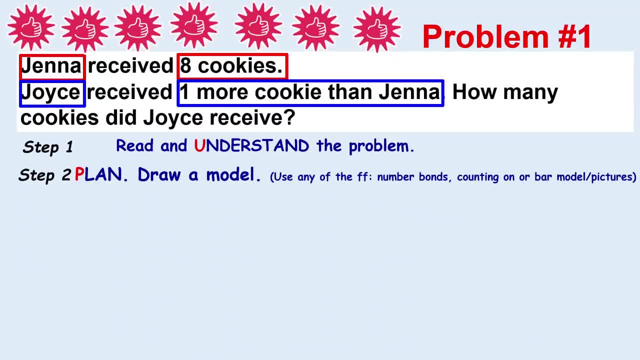 Step two, plan: draw a model. You can use any of the following: You can use number bonds, You can use counting on. We count on starting from eight. one step, so it's nine, And then we can use bar models, right. 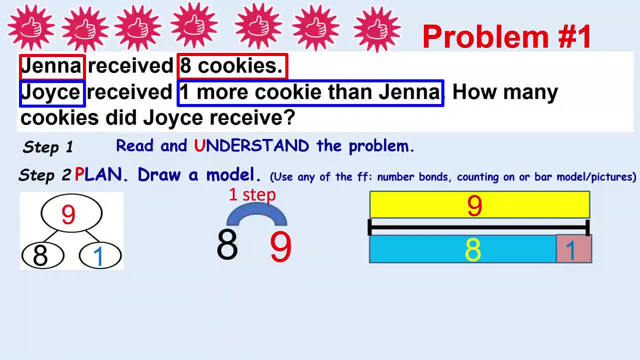 The number on top. that's the greater number. that's the total of the two parts below. One part is one, one part is eight. As you can see, the size, the different size. the greater number has the greater size. 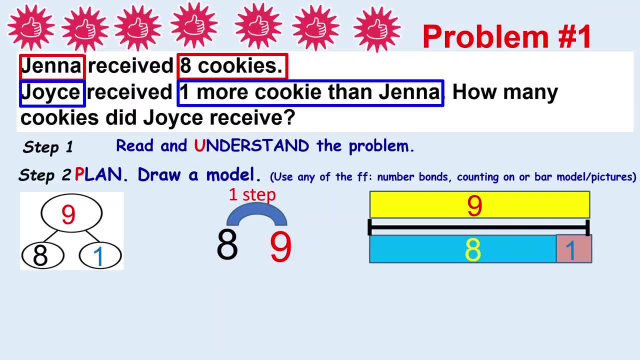 And the smaller number of course has the smaller size. So that's your plan. And then third is to solve. now Carry out the plan. Okay, write your addition sentence, So eight plus one equals nine. And then check, Look back. 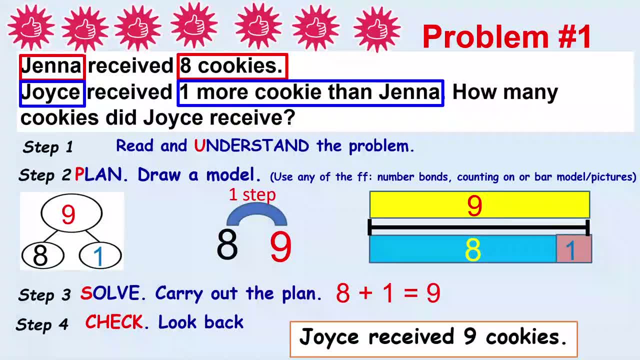 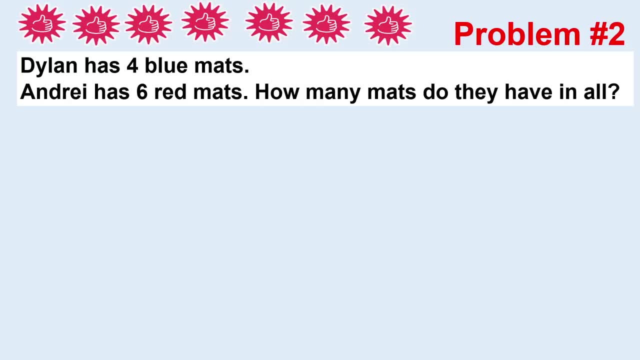 Did you solve? Did you answer the question? Yes, Joyce received nine cookies. Alright, Okay, let's have another problem. Dylan has four blue mats, Andre has six red mats. How many mats do they have in all? So let's apply. 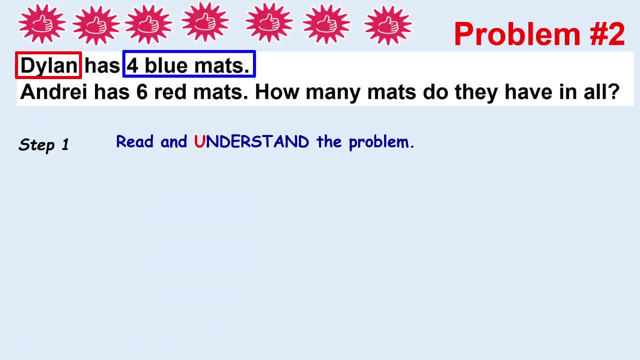 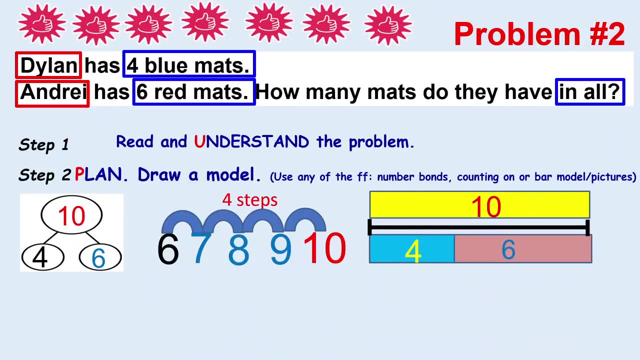 First to understand the problem. Okay, box important details, Important words or details. Yeah, you can also box in all. That means you're going to add, Then plan. Draw a model. You can use number bonds, counting on and bar models. 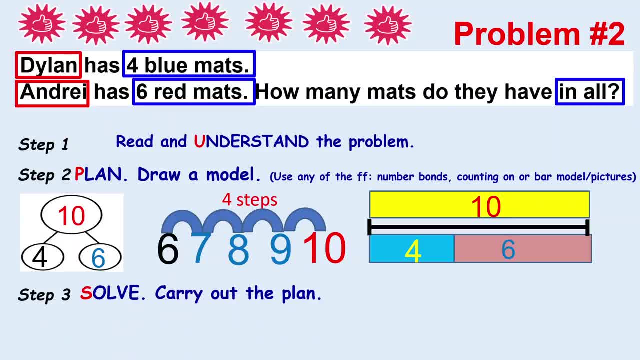 And then solve. Carry out the plan, Write your addition sentence- Six plus four equals ten, And then check. Look back, Did you answer the question? Yes, They have ten mats in all, So let's solve more problems, Alright. 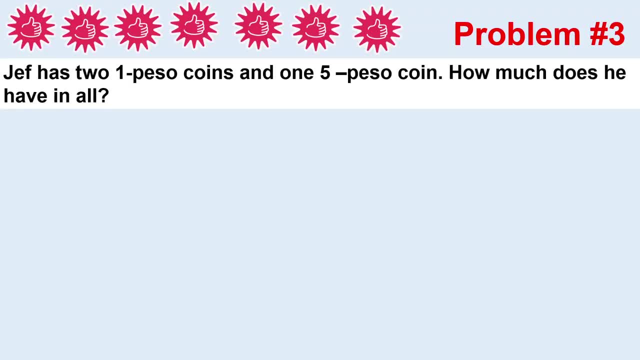 And apply UPS check. Jeff has two one peso coins and one five peso coin. How much does he have in all? How much does he have in all? So there, We understand the problem. We read with understanding Box important words, Then plan. 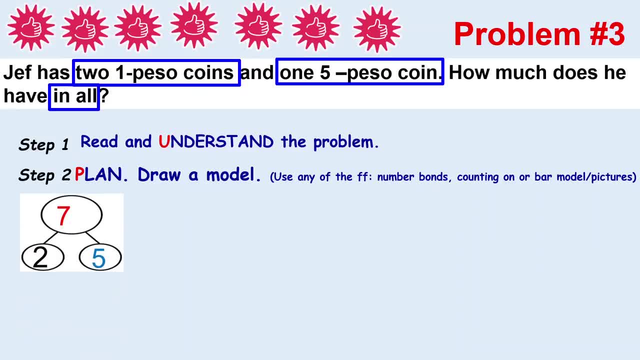 Draw a model- This can be our model- Number bonds, Counting on And bar models And then solve. Carry out the plan. There We add. We will now show the addition sentence: Two plus five equals seven And then check. 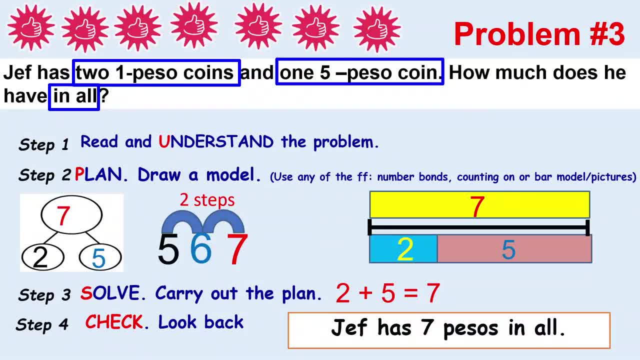 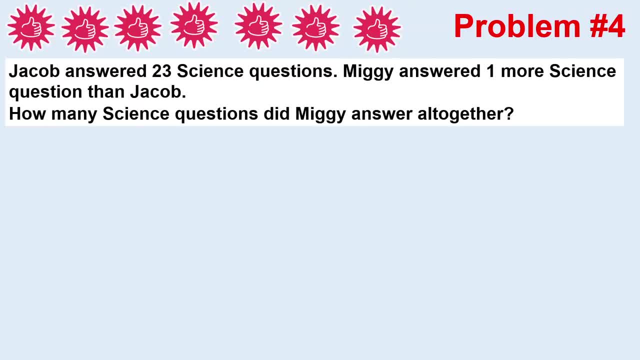 Look back. Did you answer the question? Yes, Jeff has seven pesos. in all, He answered twenty three science questions. Miggy answered one more science question than Jacob. How many science questions did Miggy answer altogether? Alright, Understand the problem. 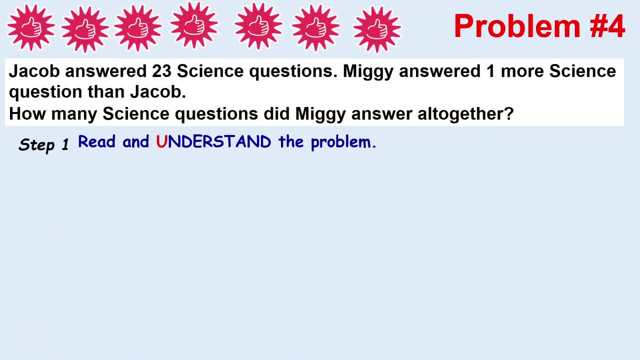 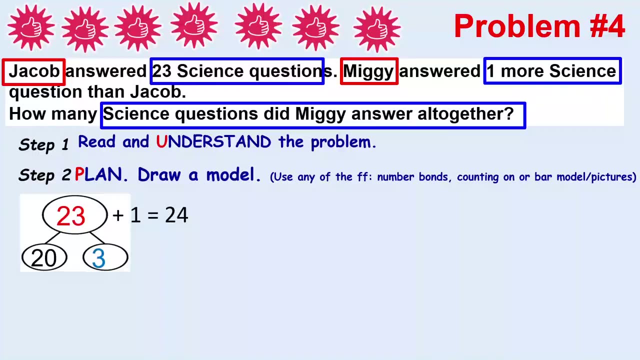 Box important details, Note them And then plan: Yeah, Draw a model. You can use either the number bonds Twenty three, That makes twenty and three, And then plan, Draw a model, And then you add one, So it's twenty four. 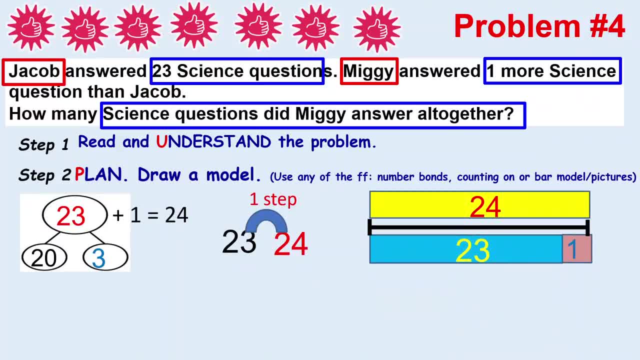 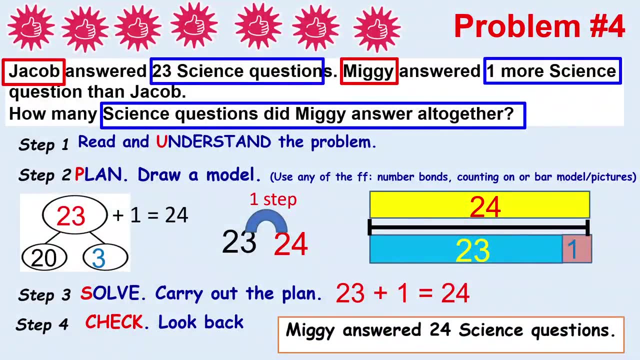 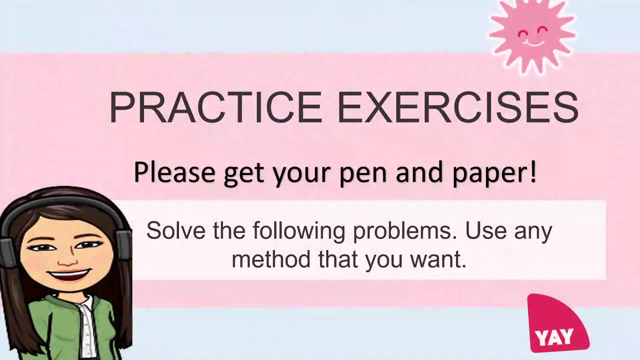 Okay, One more step That's counting on. And then bar model And then solve. Carry out the plan. now Write your addition sentence: Twenty three plus one equals twenty four, And then check. Look back. Alright, Yes, You have to do it on your own. 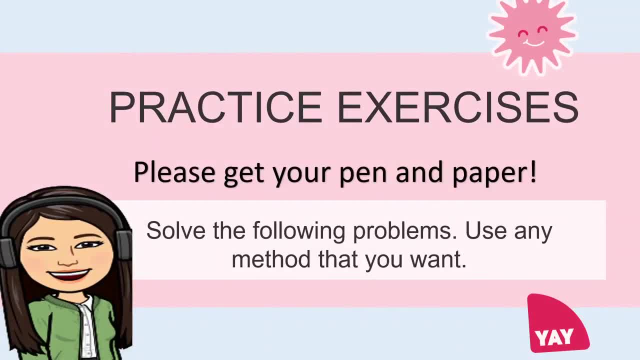 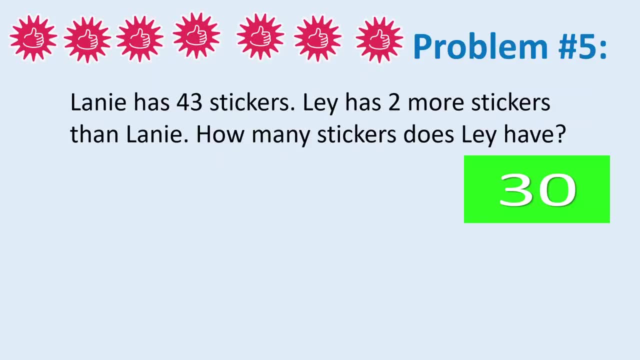 Please get your pen and paper, Solve the following problems And then use any method that you want. Okay, Alright, Thirty seconds To answer this problem. Ready Go: One, Two, Three, Four, Five, Six, Seven. 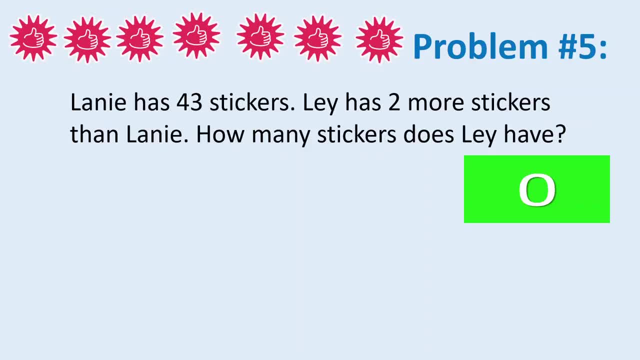